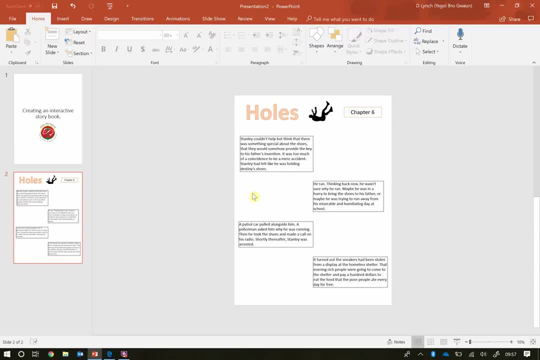 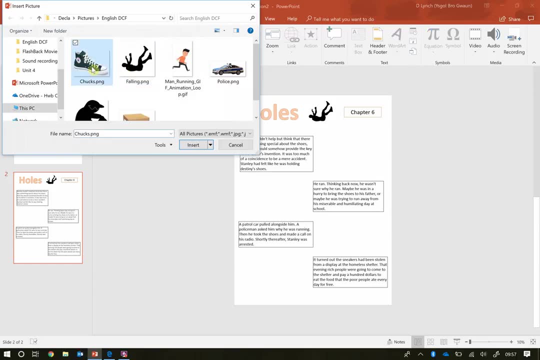 look at the first paragraph and put in a picture that could potentially link to it. So it talks about Stanley having a pair of shoes. so all I'm going to do is insert another picture of a pair of shoes. Now, what I'm going to do is I'm just going to copy and paste it. 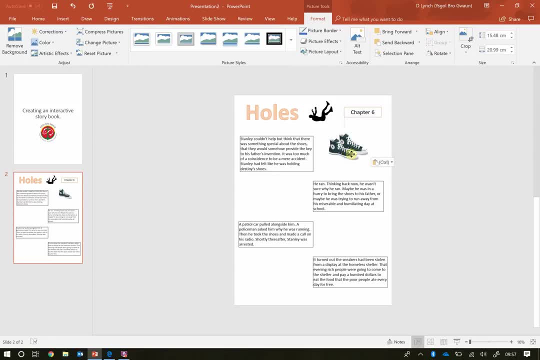 so I've got two shoes, just so it looks like a pair, and I'm going to put them next to each other. I'm then going to highlight them and I'm going to do something called grouping. Now, the grouping will just mean that you can move them as one image. 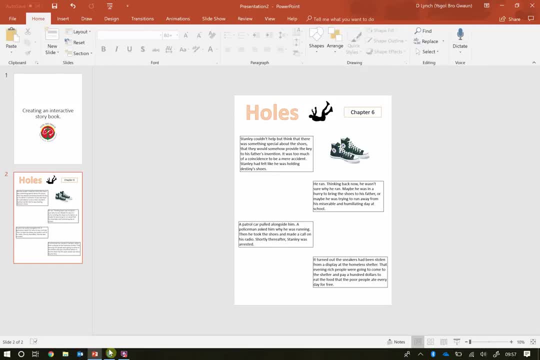 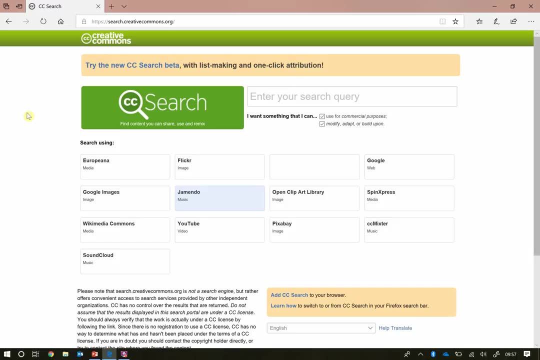 Now, all of the images that I'm using in this video today I've got from the website or I've used the search engine Creative Commons. Now this allows you to search for images that people have put up that you're allowed to use, to share, and it says here that you can use. 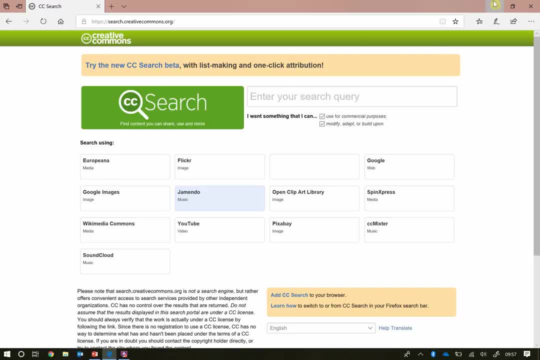 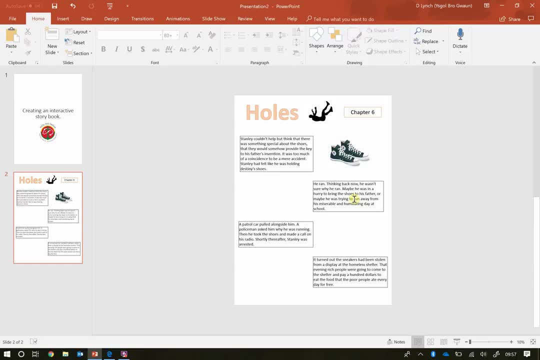 them, modify, adapt them or build onto them. Now what I'm going to do is I'm just going to completely move those images. So this is what that looks like in the next few words here. Now the next thing I'm going to do is I'm going 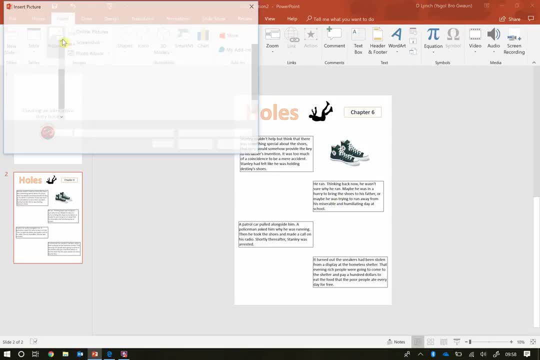 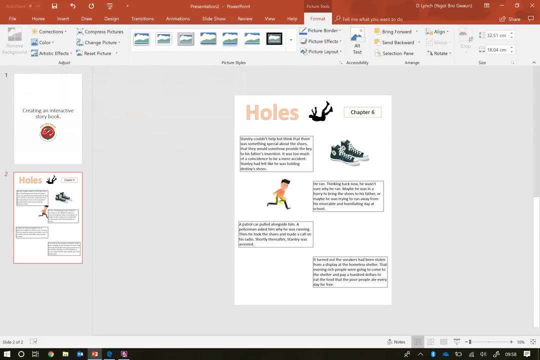 to start putting in the final few images. So it talks about someone running or he run. So what I'm going to do is I'm going to insert another picture and I'm going to put in a cartoon picture of someone running. Now, this is a gif animation or a gif image. now what this means. 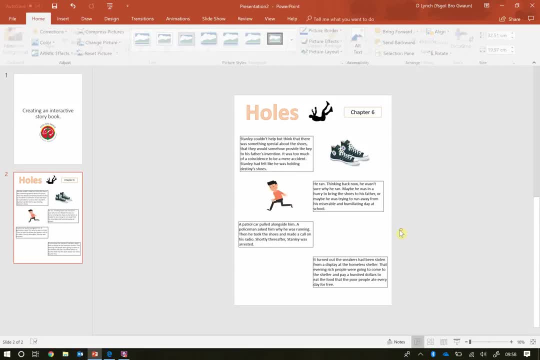 is that when the powerpoint plays, it should actually run. I'm going to turn it around just so it's the other side, final paragraphs. this one talks about a patrol car, so I'm going to insert a police car. now the police car is facing the wrong way, so I'm going to do the same thing that I did with. 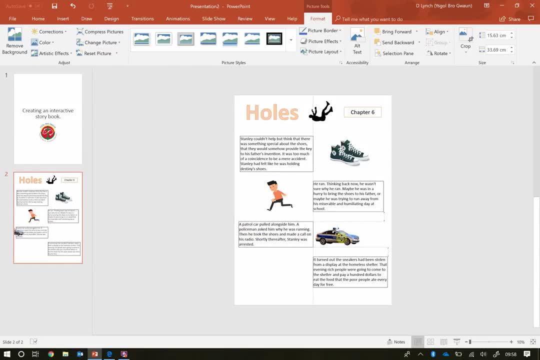 the picture above, and I'm then going to do the final one. now for the final one. it talks about the pair of sneakers. these ones at the top were stolen, so what I'm going to do is I'm going to sort of have them sitting on a table and I'm going to make it look like a robber's coming in to take them. 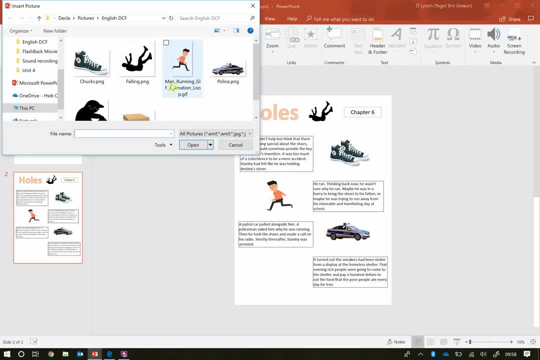 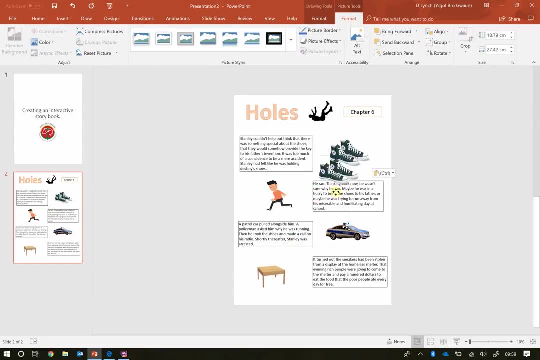 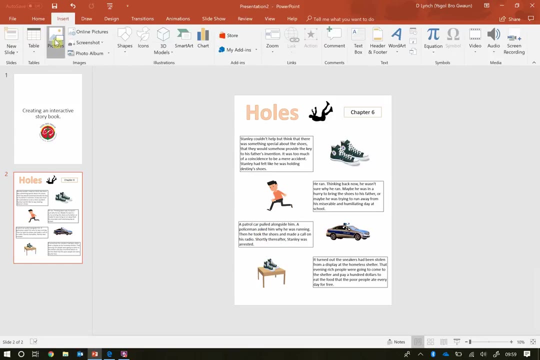 so the first thing I'm going to introduce is I'm going to put in a table. I'm then just going to copy and paste this image. so I've got two and I'm going to make it smaller just so they're sitting on the table. and the final thing I'm going to do is I'm going to insert a picture of a robber. 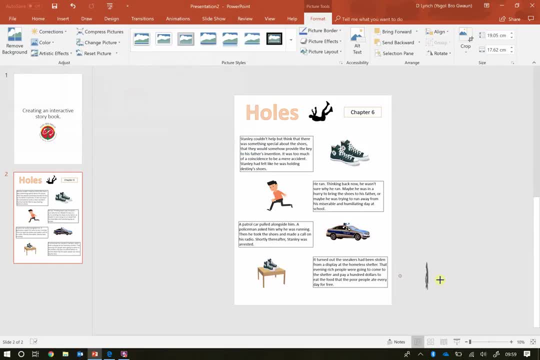 but I'm going to leave the robber just over here to start with, and I'll show you why. so now we've got all our content, basically we need to actually start making it interactive. So we need to use the animations option at the top to make them come in from different sites. Now what I'm going to do to start with is: I want 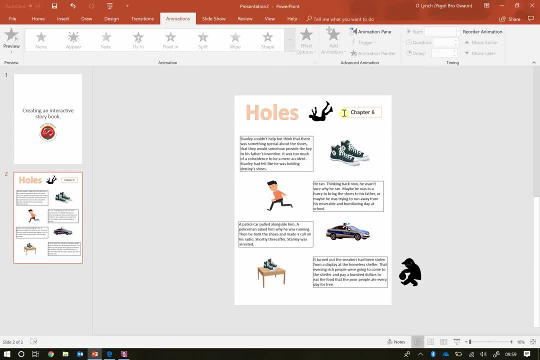 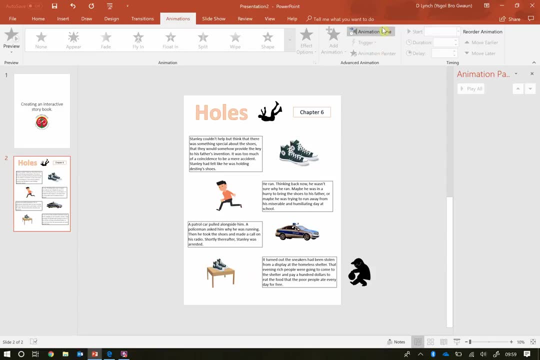 holes to already be on the page. So I'm just going to start animating chapter six and the person falling. I'm going to click this button that says animation ping. Now, what this animation ping will do is it will show you the order when you start animating things, that everything is happening. 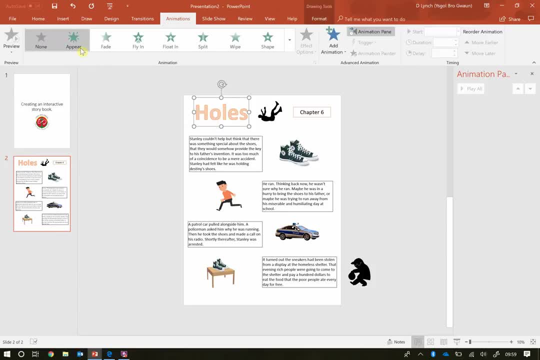 It will also put a number next to them, So I will start then with animating the holes title. It's got a number one because it's the first thing. I'm then going to click on the second or the first image that I've put in, and I'm going to use the option called fly in Now currently, as you. 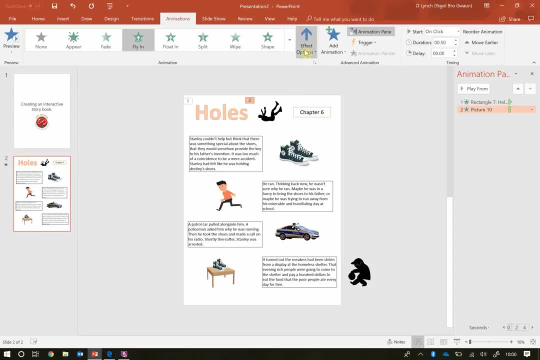 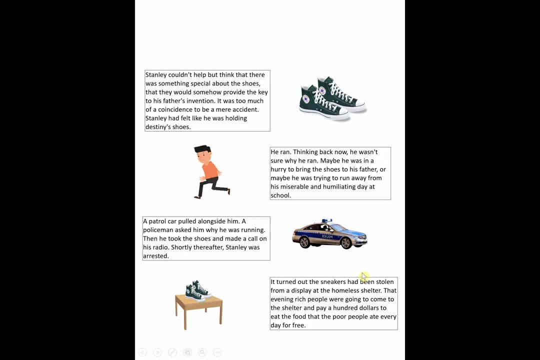 saw there, he came from the top Because he's falling. I'm going to change the effect option so he comes from the top rather than the bottom, And the final thing I'm going to do is I'm just going to animate Chapter six. Now you can always test this at any point. You can click on slideshow. You can see. 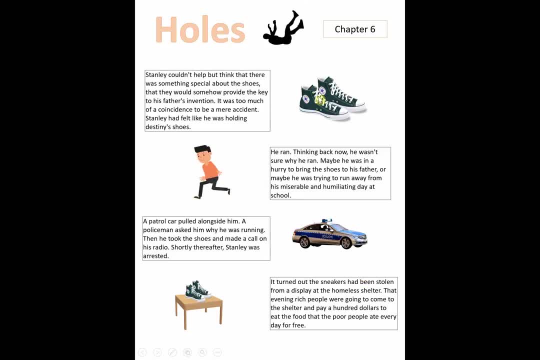 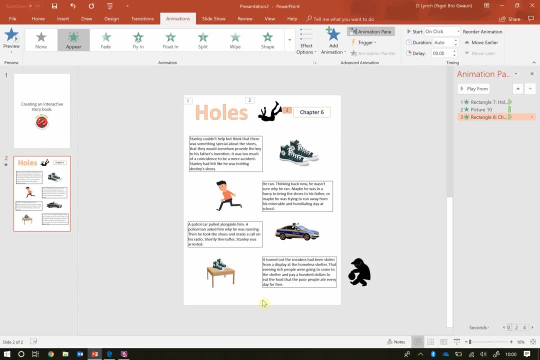 holes. You can see the person falling and the chapter. Now, because I haven't done anything with this, they already are on the page and you can see that this person is also animated, So I'm then going to start with my paragraphs. Now, all I'm going to do is I'm going to make them fly in from 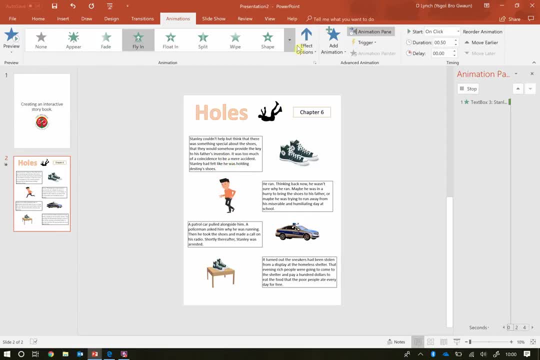 the left hand side. So I'm going to go fly in. I'm going to change the effect option from the left. I'm then going to do is I'm going to do the same with the shoes. I'm going to have them fly in. but 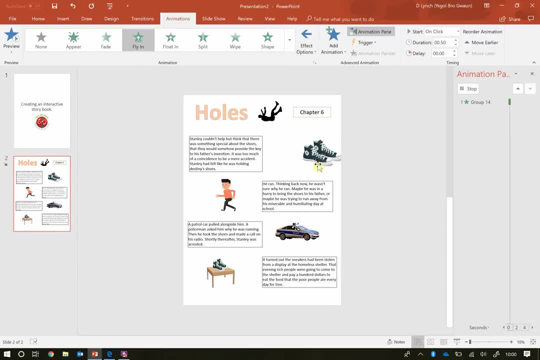 this time I'm going to have them flying in from the right hand side. I'm just going to repeat this process for the first few things. So I'm going to have this next text flying in from the right, And because this person's running, I want him flying in from the right as well. So I'm going to fly in. 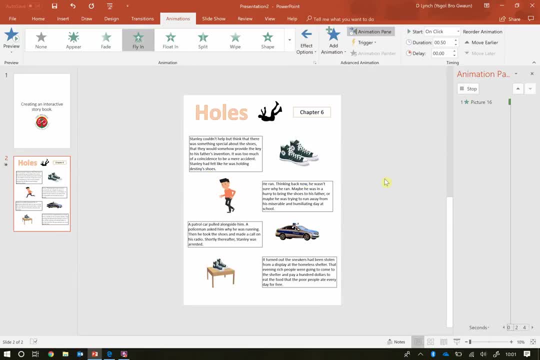 from the right. So what we saw then is, when he flew in, he actually came over the writing. Now I want him to come behind the writing, So I'm going to right click and send to back. Now that means that he then is behind the writing. I've then got my police car Now just to show you again: it comes over the. 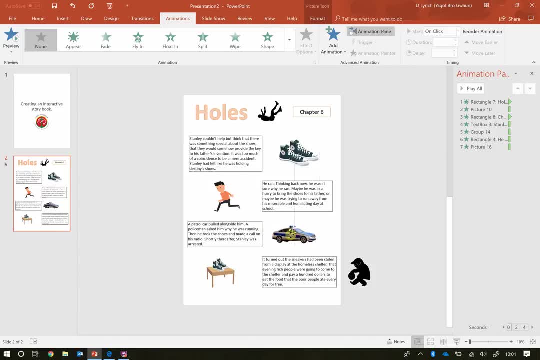 writing. So I'm going to click send to back, so it then goes behind, And then I'm going to have it flying in, And I'm going to have it flying in from the left. Now, this is where the animation pane comes in handy, because you can see that I forgot to animate this one, So I can have this one. 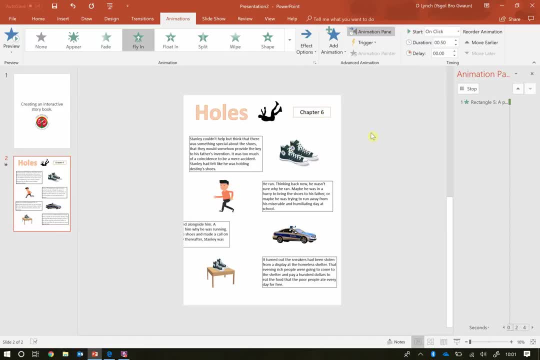 flying in. I can have it flying in from the left, And then you can actually change the order. by dragging it above, You can see the numbers change. Now the final one. I'm going to first of all group this image as I grouped the ones before, So the table and the shoes move as one, And I'm then 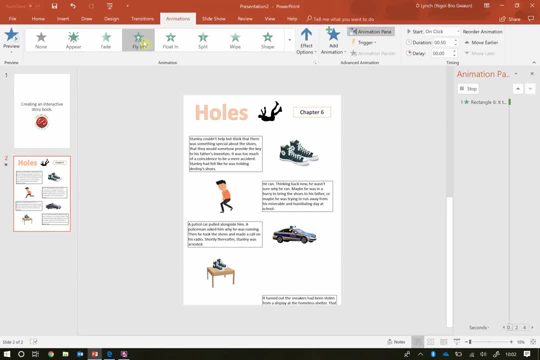 going to start animating it. So the first thing that I want to happen is I want to have the final piece of text And I can have that flying in from the bottom, because it's the bottom of the page. I've then got the shoes on the table And I'm going to have them coming in from the left. 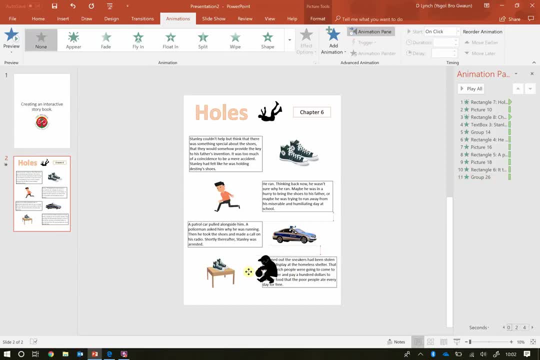 hand side, And I've then got the robber. Now I'm going to have him sent to back, But what I'm going to do this time is, rather than just having him come across, I'm going to use something called a motion path. Now, a motion path will allow me to make him come in at whatever angle I want him to. Now to do this. I'm going to have him come in from the left And I'm going to have him come in from the right, And I'm going to have him come in from the right And I'm going to have him come in from. 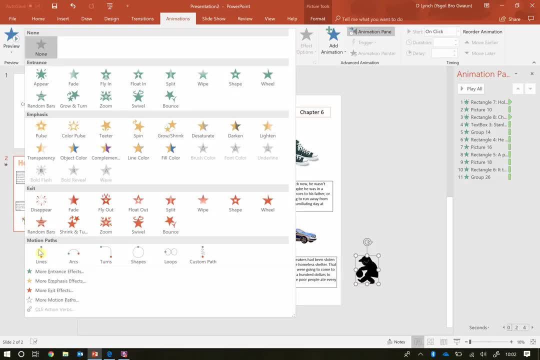 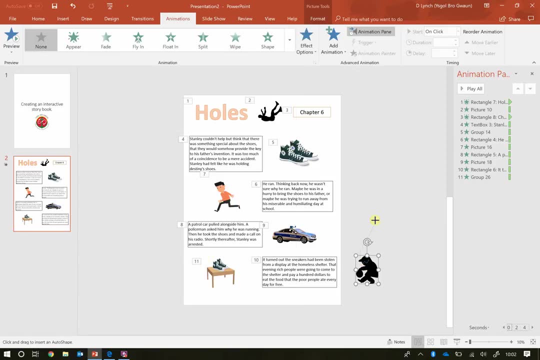 this angle. Now, to do this, I'm going to go on add animation When I'm going to look at the motion path options here. I'm then going to click custom path and this means that I can then click and I can draw the path that he takes. I'm then going to double click to finish my animation. Now what? 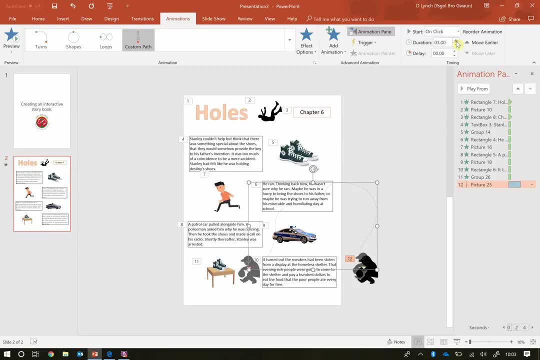 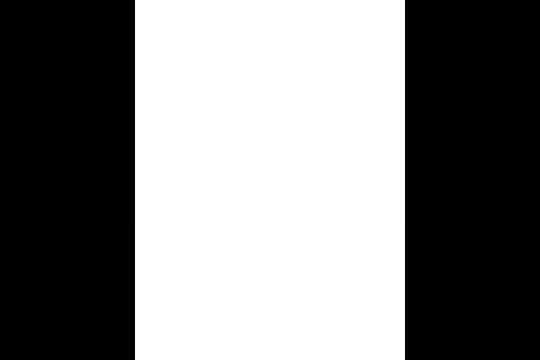 you did find there is. he came in quite quick. So what I can do is I can change the timings at the top to make the animation last slightly longer. If I then go and I run through my animation, I've got the title and the chapter and then.